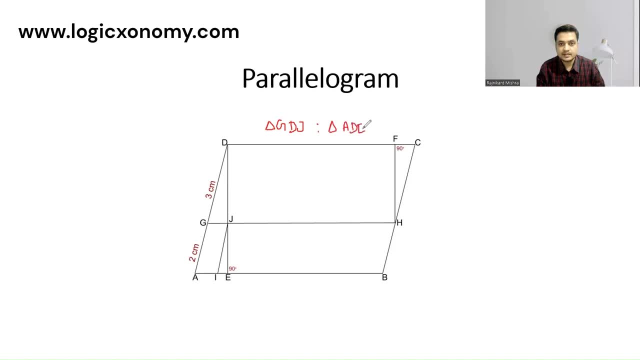 D, E, A D E is equal to D, G square ratio: A D square D G is 3, square A D is 5, square means 9, ratio, 25.. So we can put area of G, J, D as 9 unit and area of body literal A, E, J. 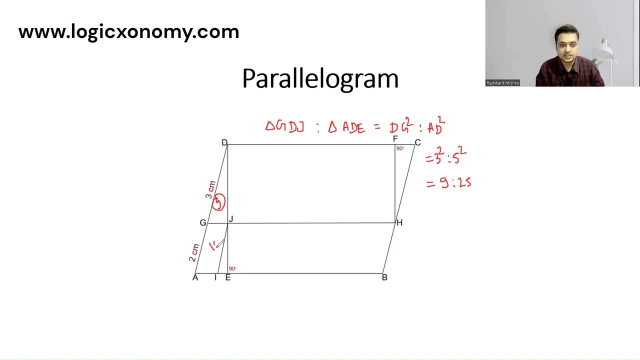 G is 25 minus 9 is equal to 16 unit. Now compare triangle G, J, D and I E J. Here angle I is equal to angle G. Here this angle is 90 degree. This angle is 90 degree. So 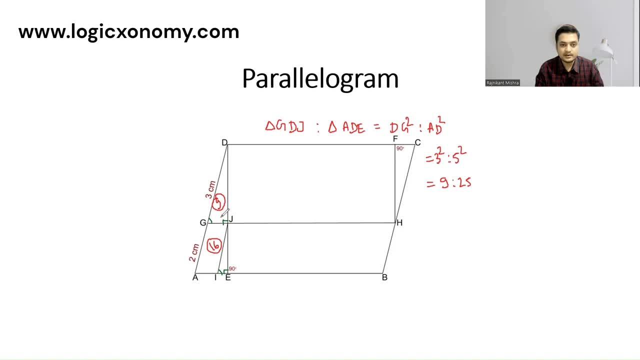 both the triangles are similar triangle. So compare the area of G J D, Area of G J D ratio, area of I E J D G square ratio. I J square D J is 3 square, I J is 2 square means 9 ratio 4. Here. 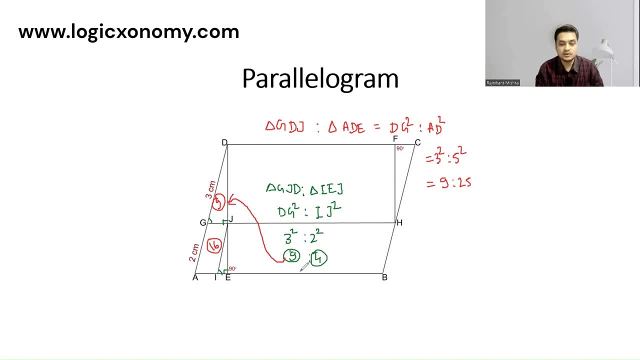 this 9 and 9 equal means 1 unit is equal to 1 unit. So area of triangle I E J is 4 unit. So area of triangle I E J is 4 unit. So area of triangle I E J is 4 unit. So. 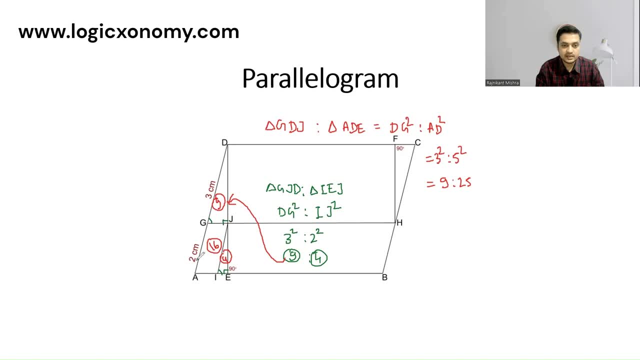 now we can say: area of body literal A, G, J, I. Body literal A, G, J, I is equal to 16 minus 4 is equal to 12 unit. Now see triangle G, J, D is congruent to triangle H, F, C because D, J is. 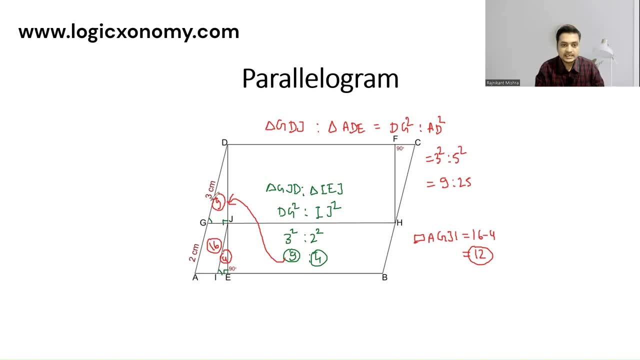 equal to F, H and D, G is equal to C, H, And this angle is 90 degree, common in both the triangles. So if this is 9 unit, then the area of triangle H, F, C, also 9 unit. Now the ratio of these two areas, this 12.